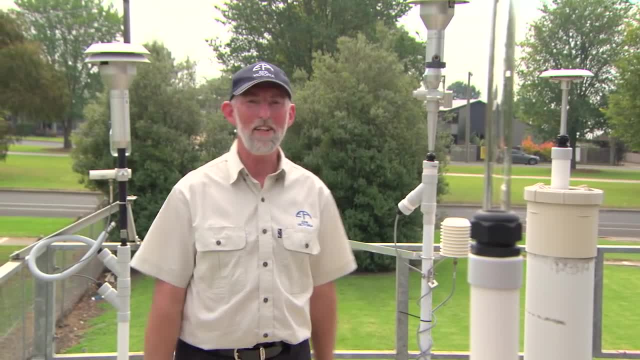 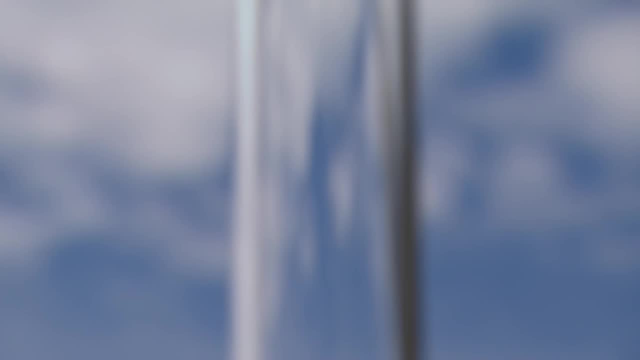 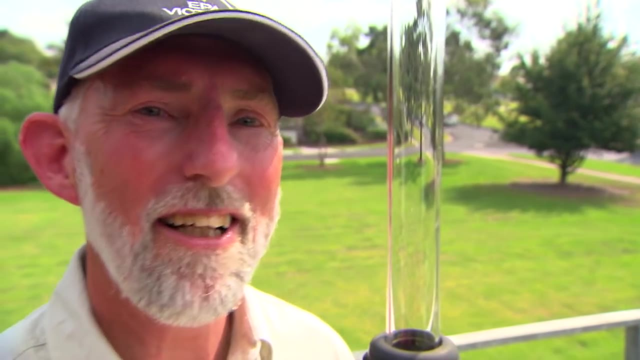 On the roof of an air monitoring station, you can see a number of inlets. These inlets are connected to instruments inside the station. This class inlet is connected to a number of instruments which measure gases such as ozone, carbon monoxide, sulphur dioxide and nitrogen. 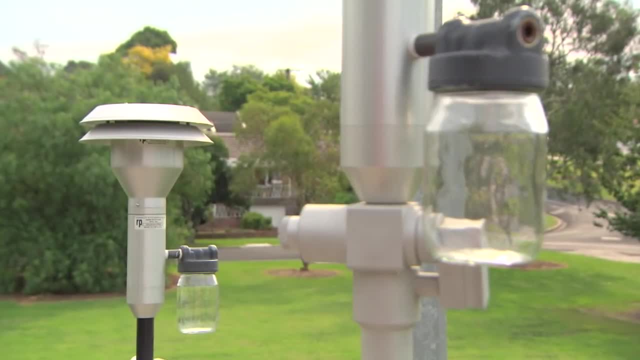 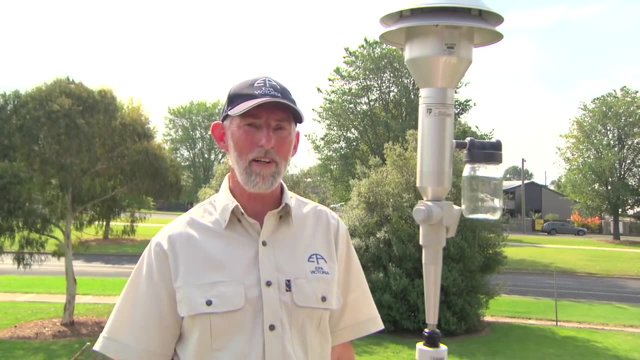 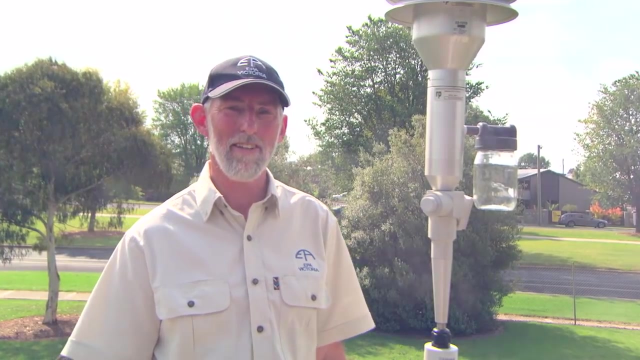 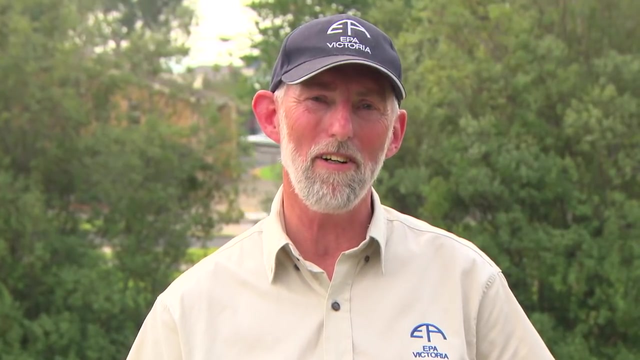 This inlet draws in air to measure particulate matter 2.5 or PM 2.5.. The concentration of PM 2.5 is one of the more important indicators of healthy air. PM 2.5 particles are extremely small particles present in smoke and in some fine dusts. 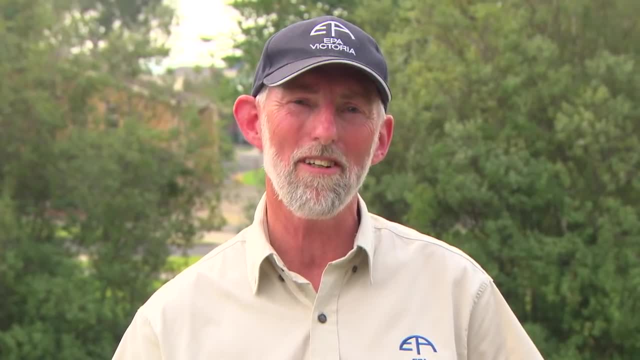 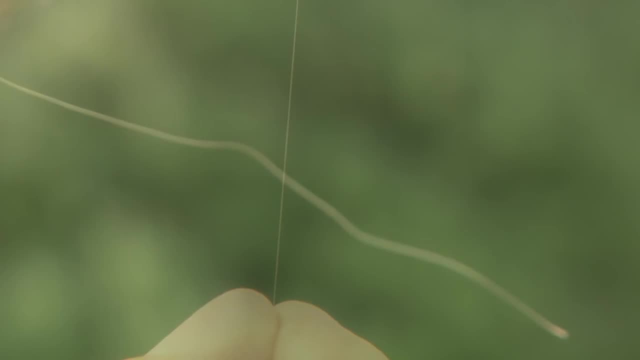 They measure 2.5 micrometres or less in dioxide. To give you an idea of how small that is, a strand of hair is about 75 micrometres in diameter, So these particles are over 30 times smaller than that. 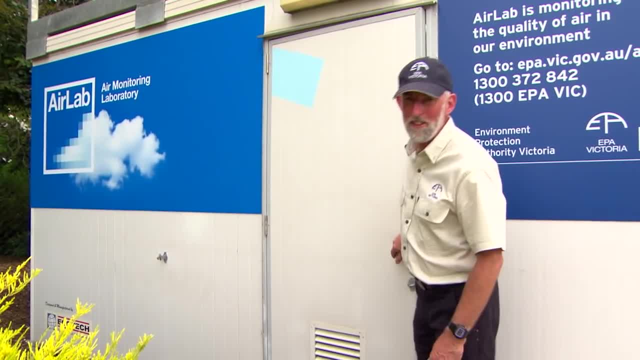 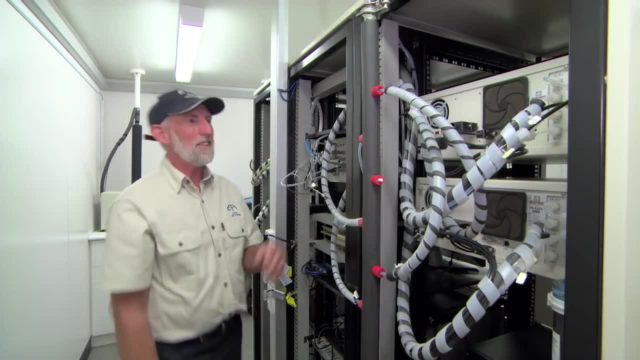 I'm going to take you into the station now. It can be a bit noisy because equipment has to run 24 hours a day. This is connected to the glass inlet we saw on the roof. An air sample travels down and is distributed to the various analysers. 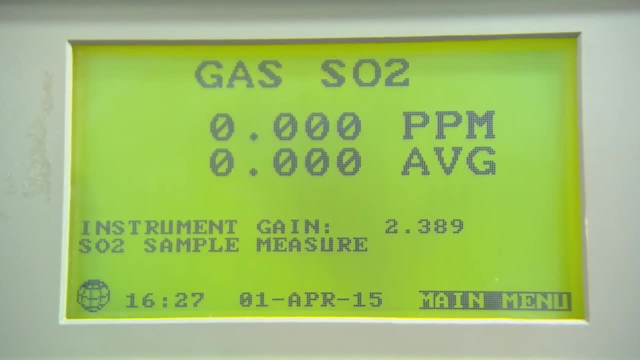 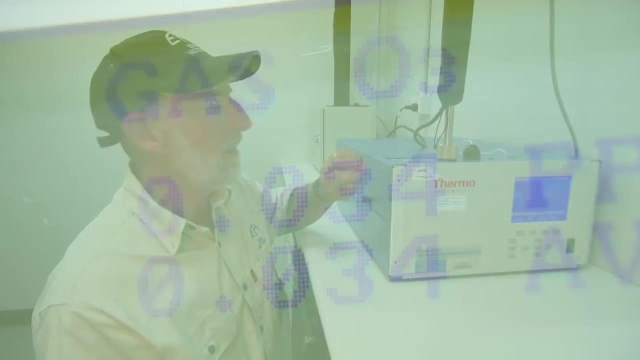 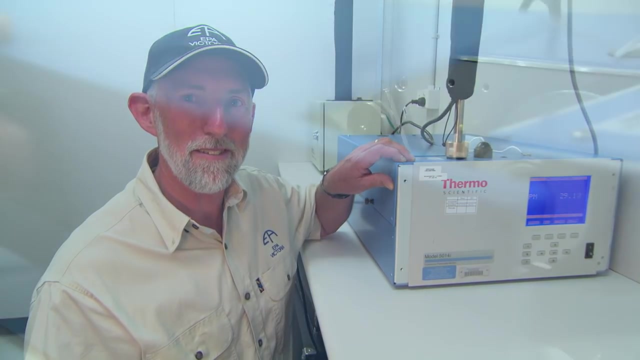 Each one of these measures a particular gas: Sulphur dioxide, carbon monoxide, nitrogen dioxide and ozone. The instrument here is a beta attenuation monitor. It measures those tiny particles I mentioned earlier. Inside this instrument is a roll of tape. The particles which come down the inlet are deposited on the tape. 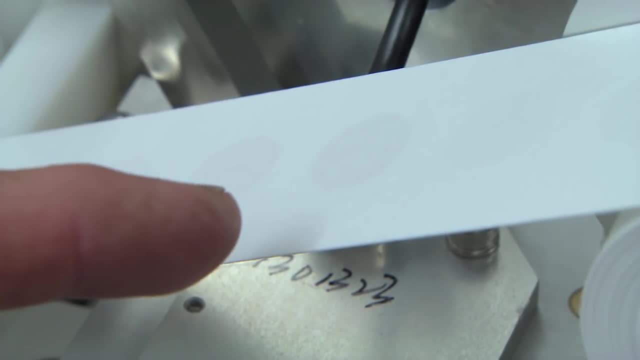 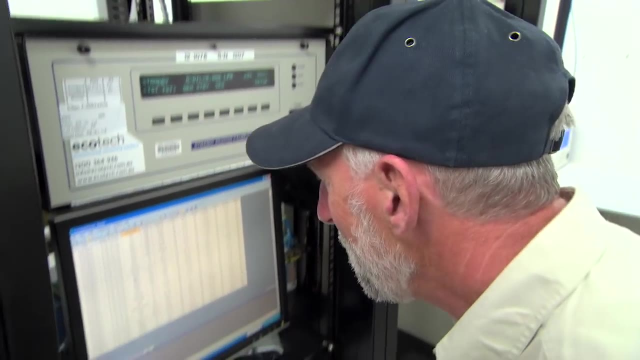 As you can see, when these tiny particles land on here, the tape can sometimes change colour. All the air quality data collected by the different types of instruments inside the air monitoring station is sent to this computer 24 hours a day, 365 days of the year. 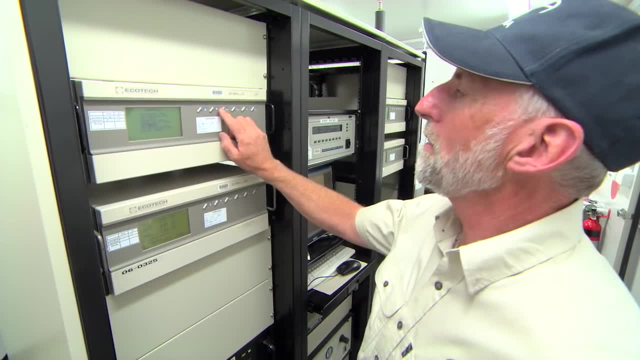 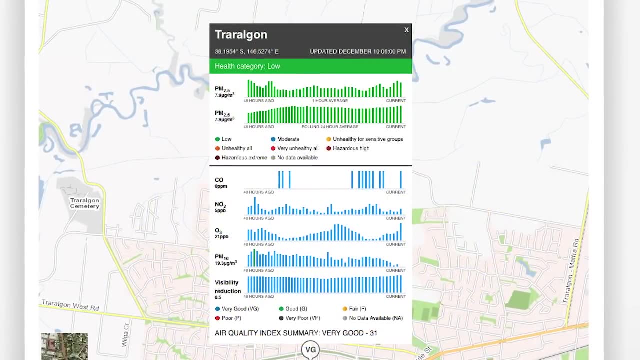 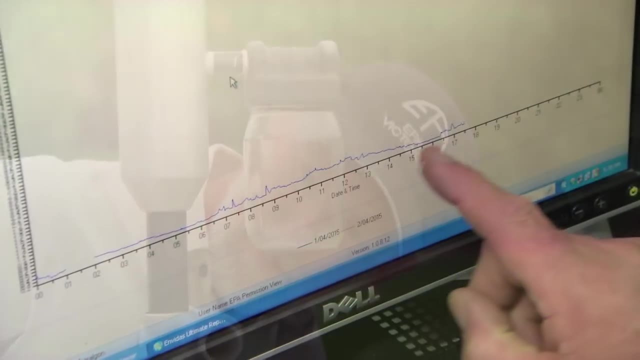 From here the data is sent to our computer and then goes up on the EPA's website. EPA scientists also use this data to prepare daily air quality forecasts. EPA has been monitoring ambient air quality in Victoria since 1979.. Technology has come a long way since then, and so have we.